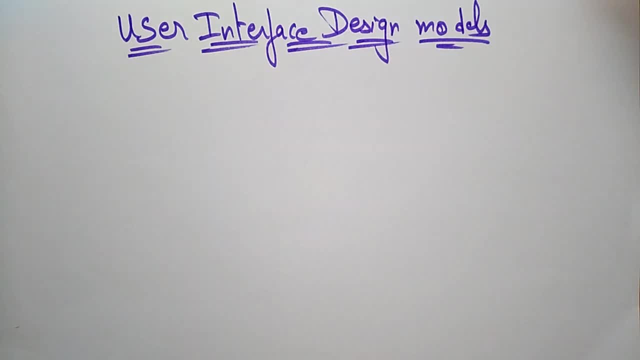 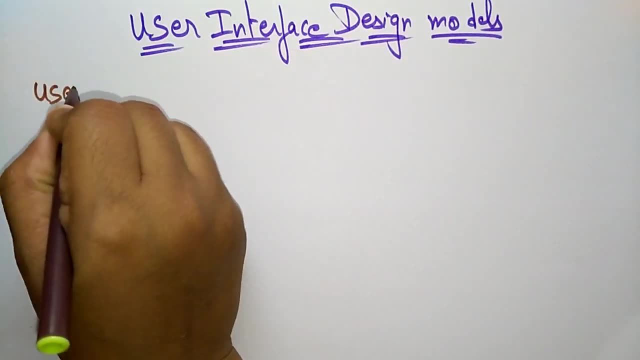 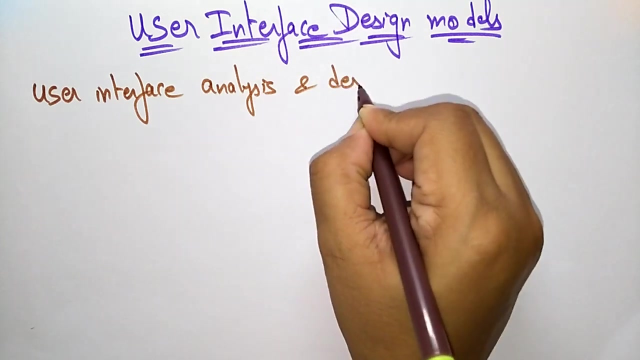 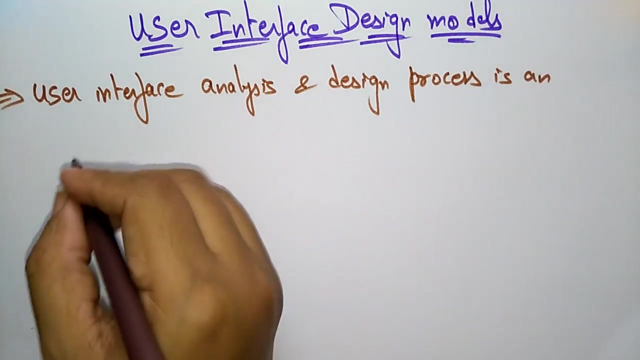 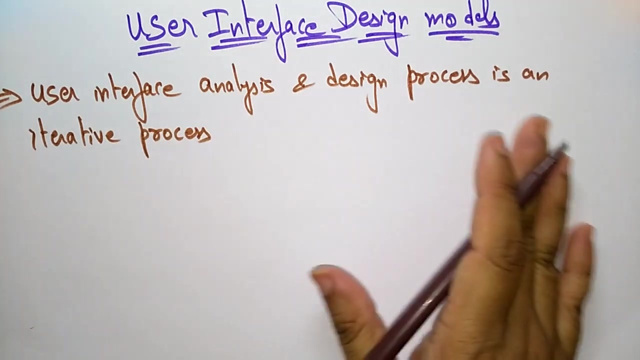 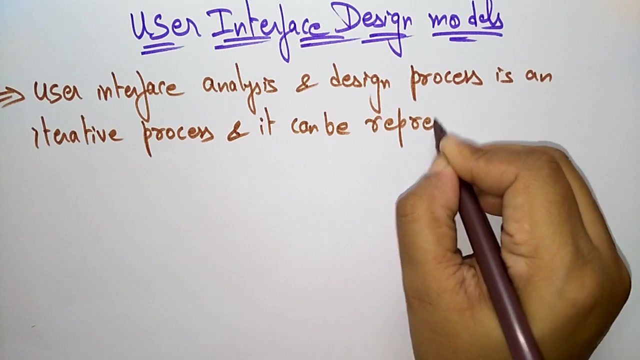 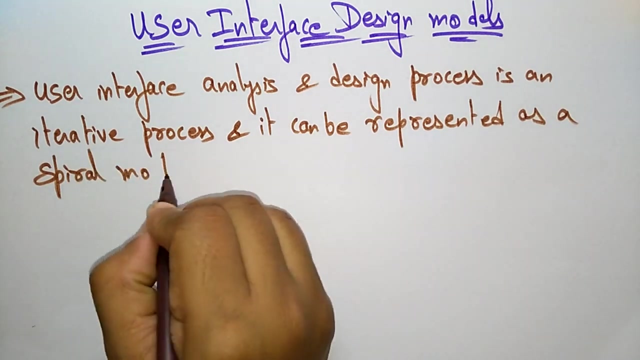 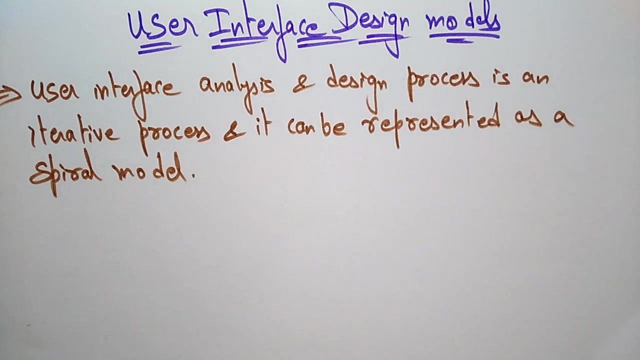 Now let us see what this user interface and analysis. let me explain with this example User interface analysis and design process. First, it is an iterative process. So the user interface analysis and design process, So the user interface analysis and design, will follow the iterative process and it can be represented, And it can be represented as a spiral model. So this iterative process will be represented by using the spiral model. Actually, this user interface analysis and design consists of. it consists of: 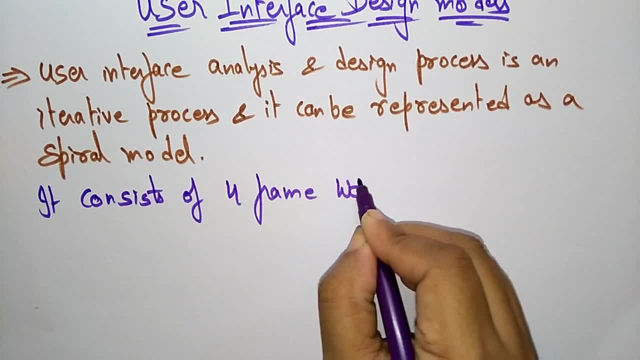 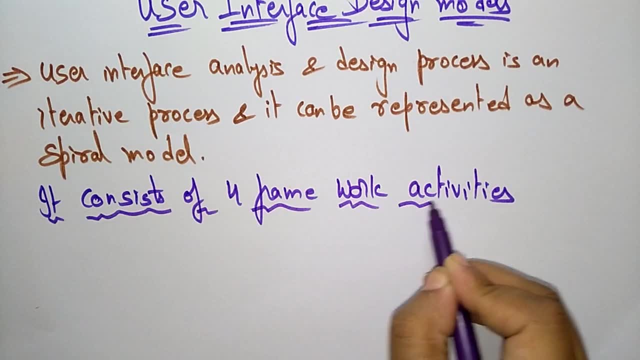 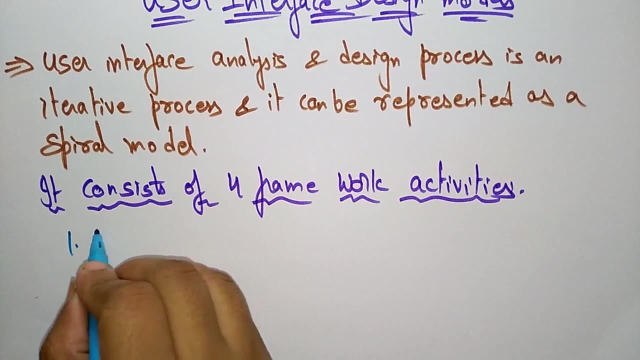 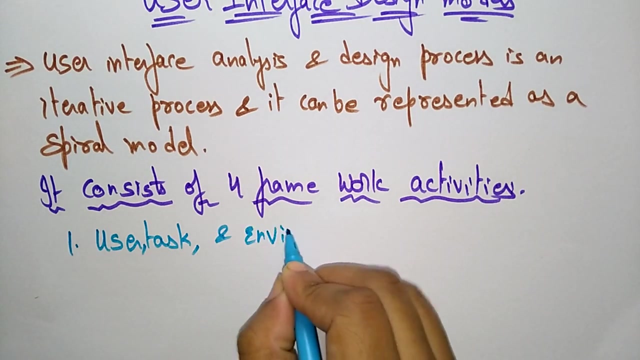 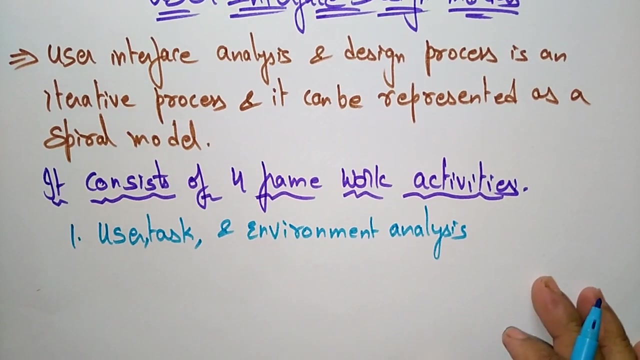 Four framework activities, Four framework activities. So what are those four framework activities that are present in the user analysis and design, which are represented in a spiral model? So the first is user task means user task and environment, or Environment or interface analysis. So the first framework is user task and environment analysis. 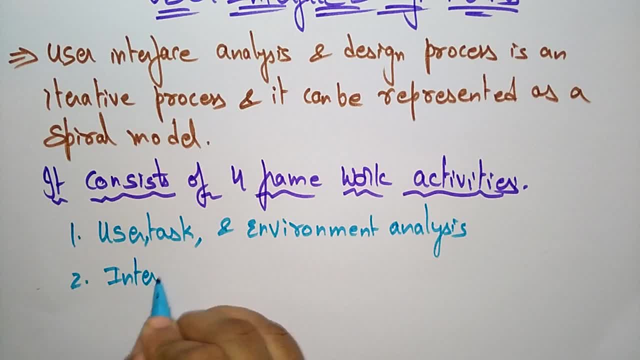 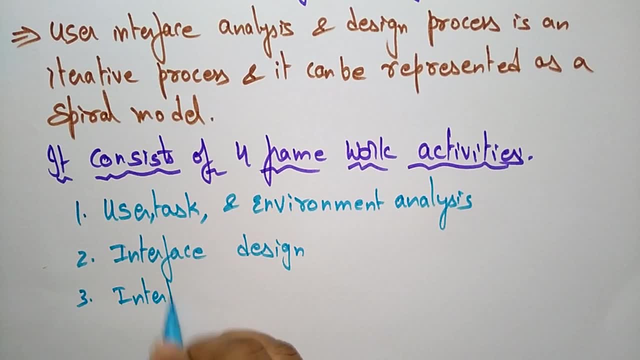 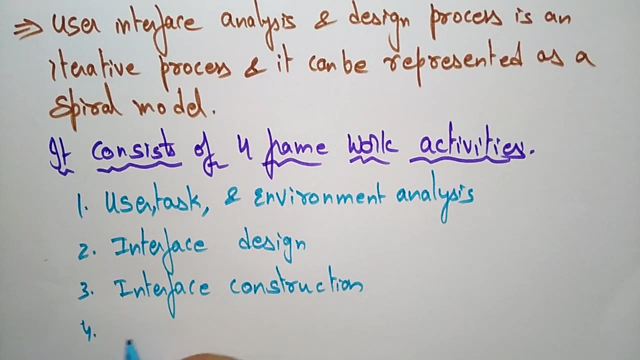 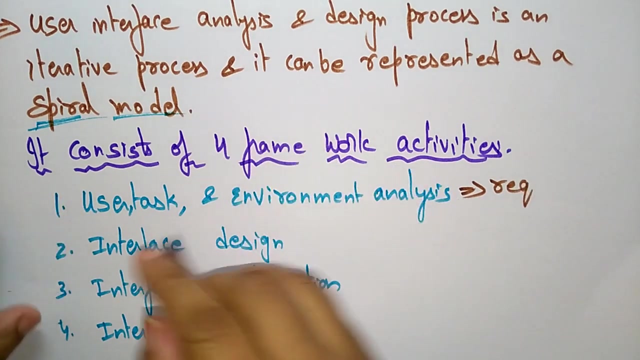 Second activity is Interface design, Next, interface construction, or you can call it as implementation. And the fourth one is in interface validation. So these are the four Framework activities which are represented in the spiral model. means the user interface. If you want to analysis and design the user interface process, you have to follow these four framework activities. First, you have to use it, You have to gather the user task and whatever the task that the user is giving. and the environment analysis means the interface analysis, that you are going to gather the requirements. So in this framework, 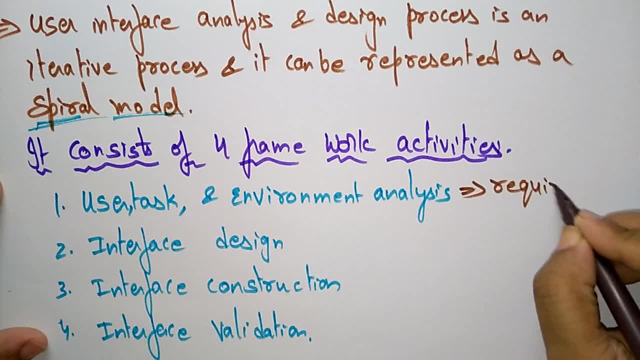 Okay, in this Framework, we are gathering the requirements, Requirements Gathered And in the interface design, we are going to find out the objects You have to design. Design the framework in the way that you have to find out what are the objects that we are using on that process. 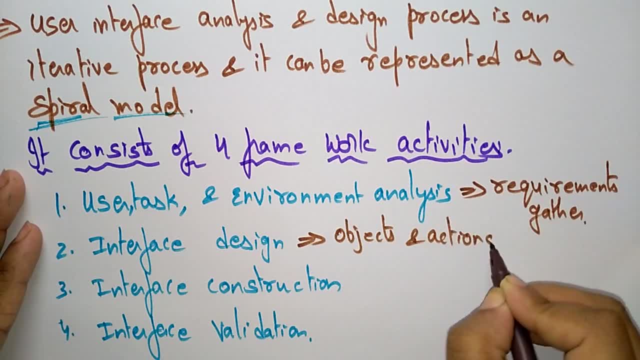 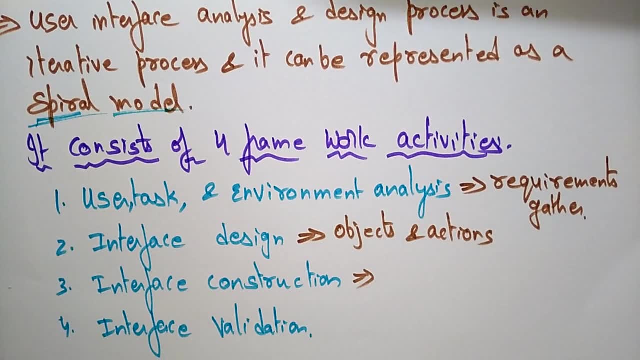 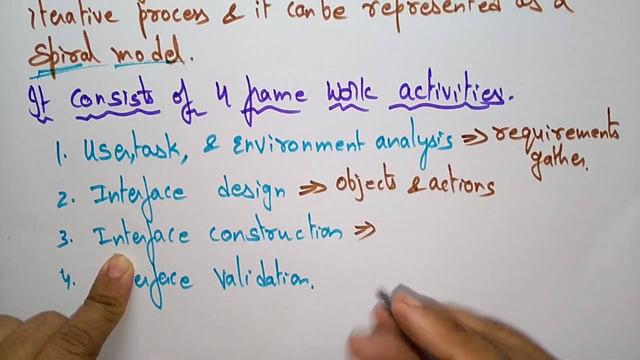 Okay, and actions that we are going to be taken place, so that will be represented in the form of a design. So that activity is an interface design. So, Okay, I, I designed, whatever the process that I want to be implemented. Next is the interface construction. So, after designing, we have to construct. 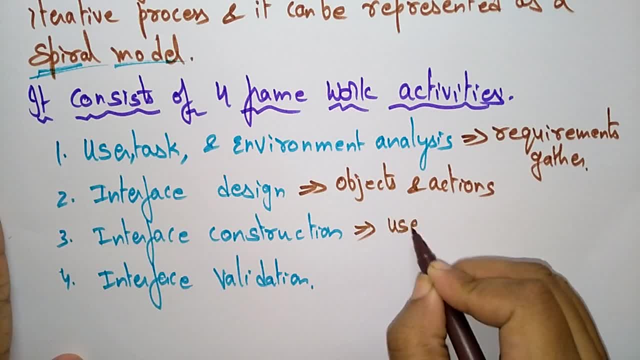 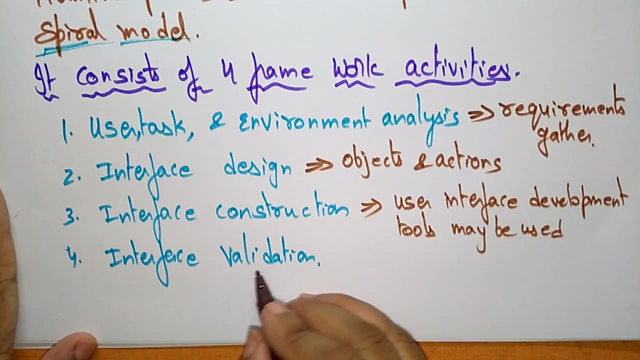 So here, in this construction framework, user interface Development tools may be used. Development tools May be used in this interface construction. And finally, this is A The last activity that we have to be done is the interface validation. So this interface validation will correctness of 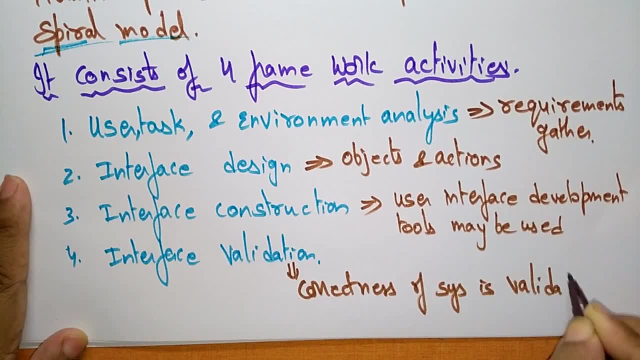 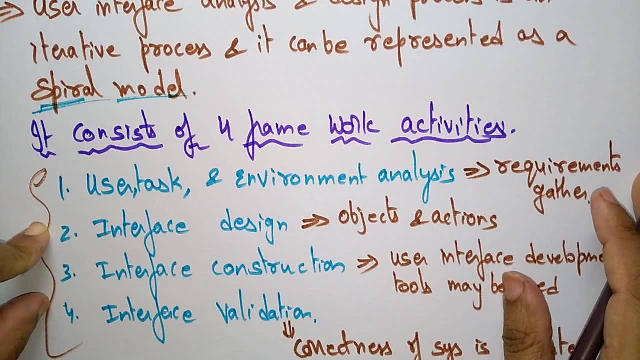 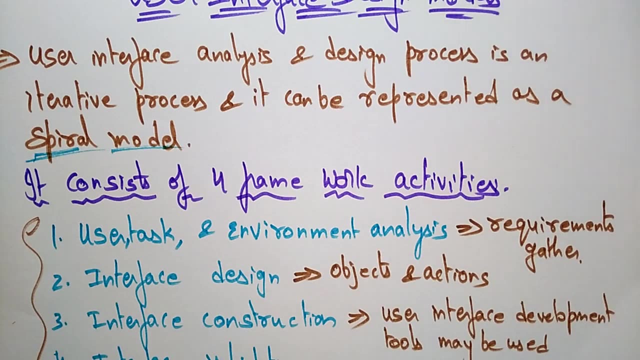 System is validated here. So these are the four framework activities that we have to be performed in a user interface analysis and design process. So here I'm just explaining. already I explained the design model, So the design is a user model, design model. 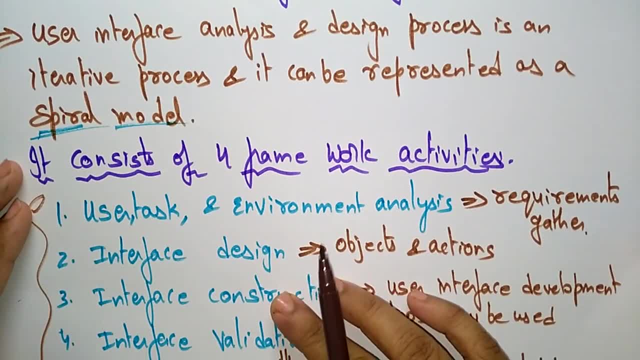 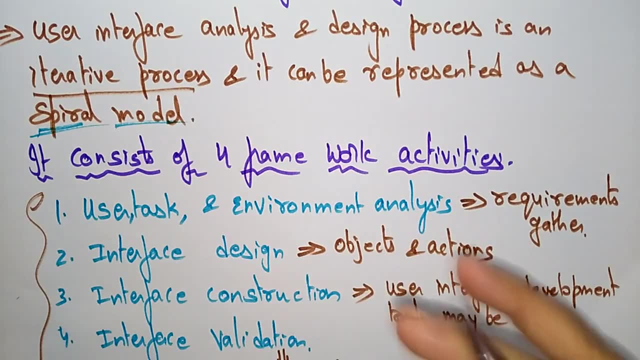 Mental model, An implementation model. Everything is the same here, Okay, but here the main thing is we are representing. everything means the process is done in. here, in iterative process, We are following one of the process by taking that four design models. So these are all the four design models. 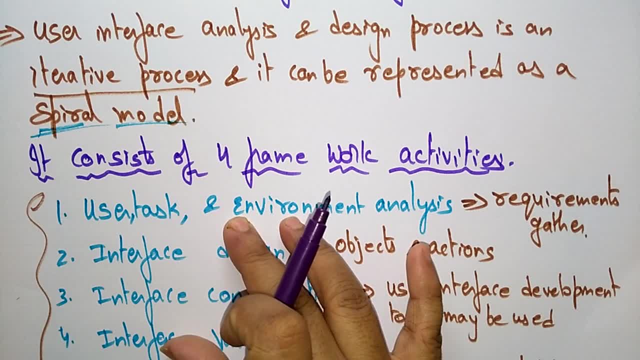 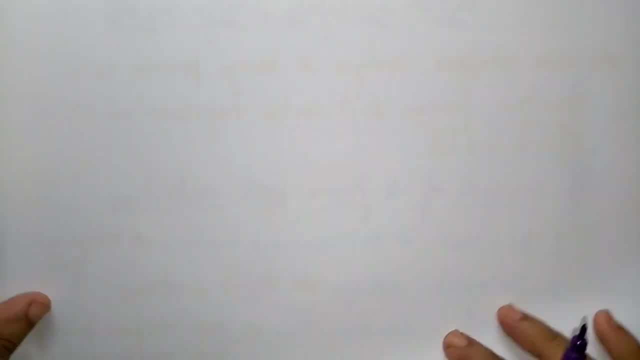 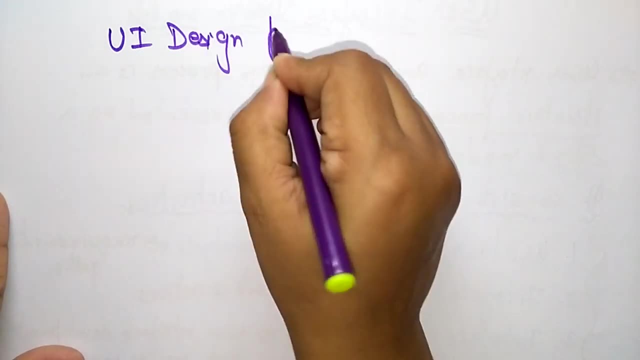 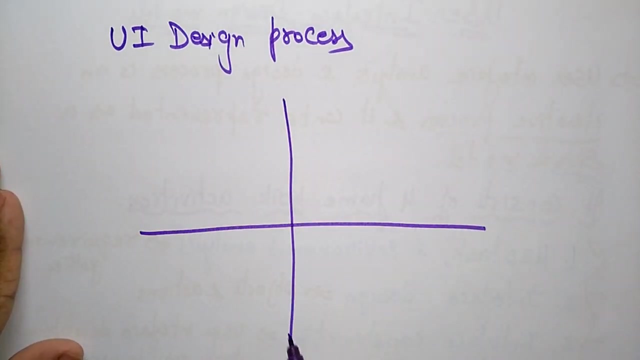 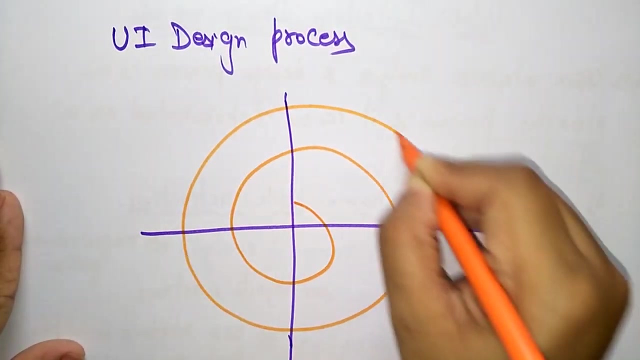 So these four design models Are executing in the form of iterative process and it can be represented as a spiral model. So the spiral model can be represented as A User interface. Design Process can be represented in spiral model. Okay, so what face is this? 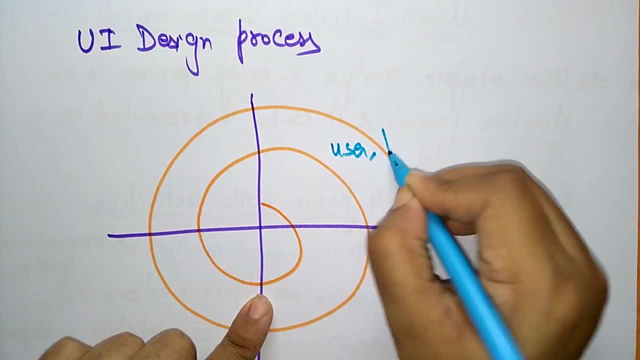 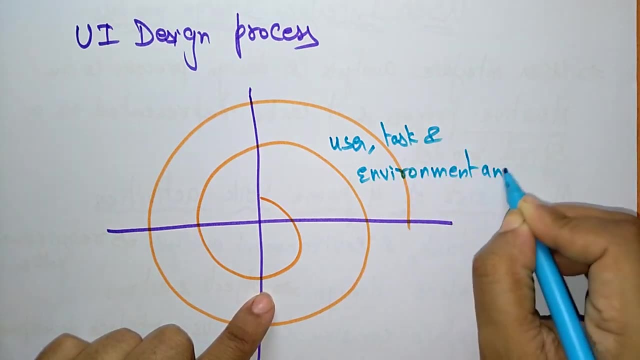 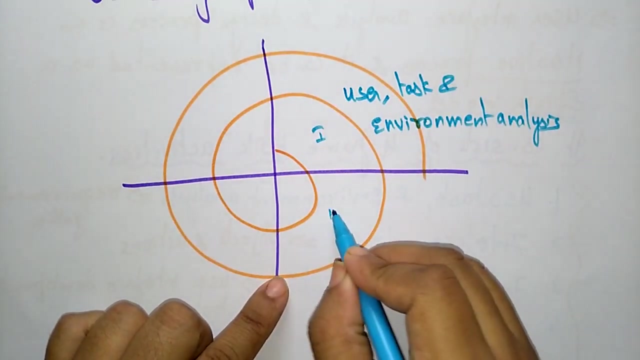 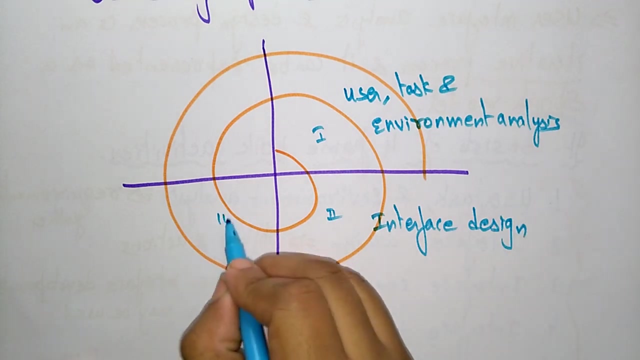 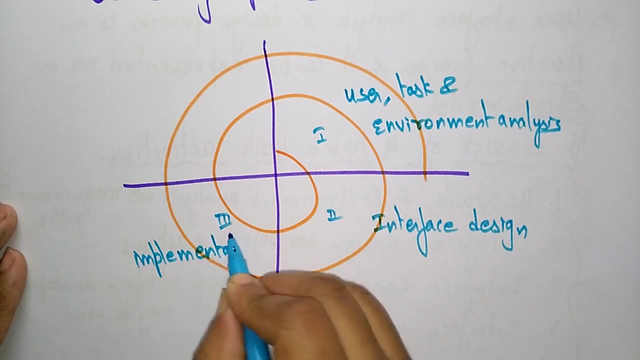 So here the user Task And environment analysis phase, Okay, So. So this is the first task. So here are, requirements are gathering, and next is, in the second task, interface has to be designed. So in the third task we will going to be implement or construct the process.